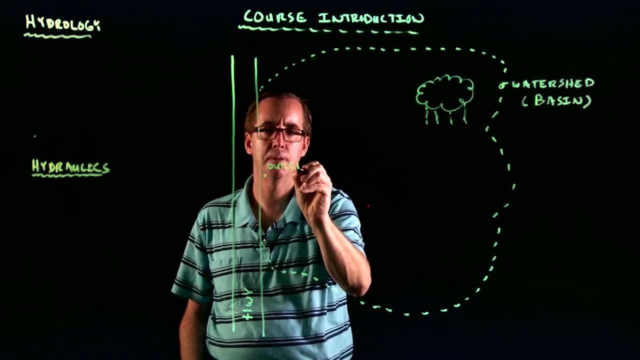 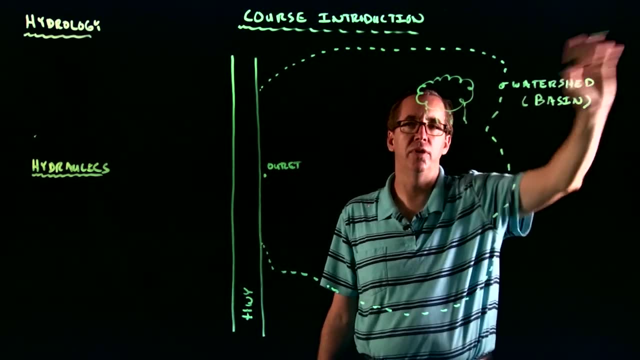 that we call the outlet. Okay, If there is a drop of rain outside this boundary, then it would basically go on in a different watershed. So again, the watershed is kind of bounded by. it's a region in which a watershed is going to be in the same direction as the watershed is going to be in the 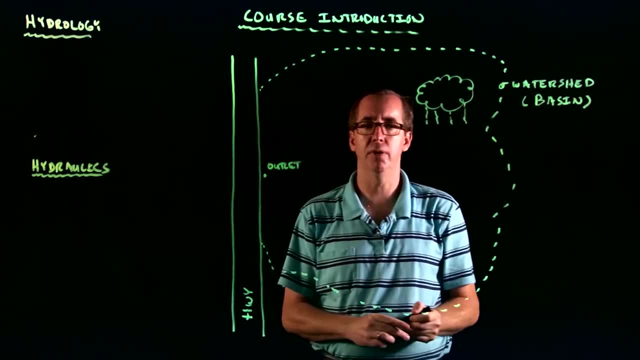 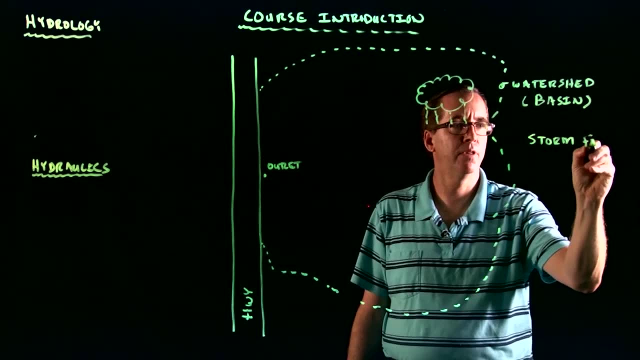 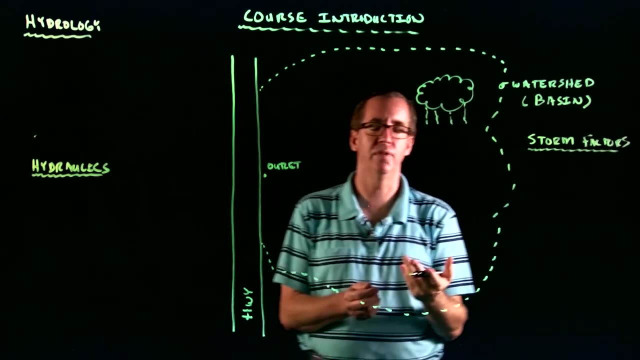 same direction. Any rainfall within that region makes its way to a single outlet. Okay, Now you know, talking about rain, there's lots of different factors that influence the precipitation, Okay, Or kind of characterize the precipitation. The first thing we need to talk about is the duration. Okay, 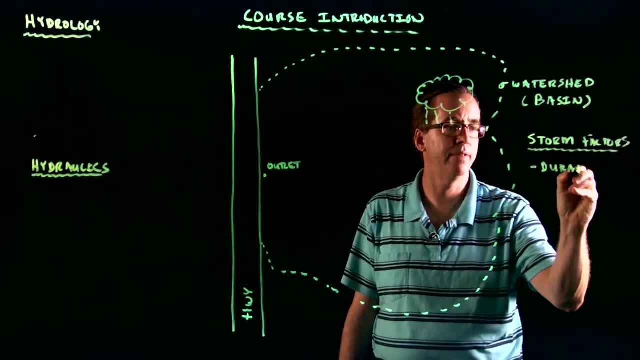 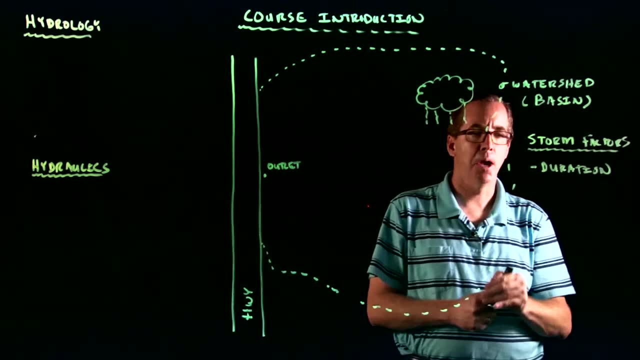 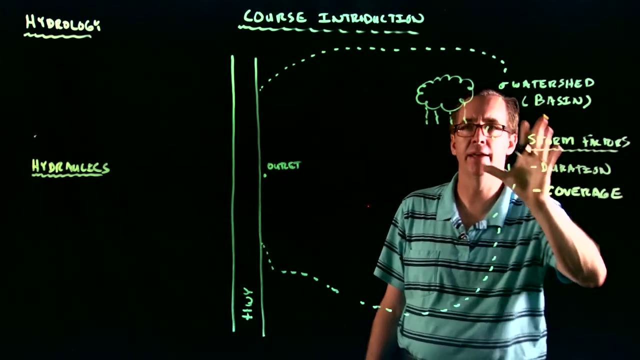 Is this a storm that's a matter of minutes, Or are we talking about a storm that lasts hours? Okay, Let me switch markers. Another issue that we have to consider is the coverage of the storm, And what I mean by that is: is the rain only affecting this part of the watershed? 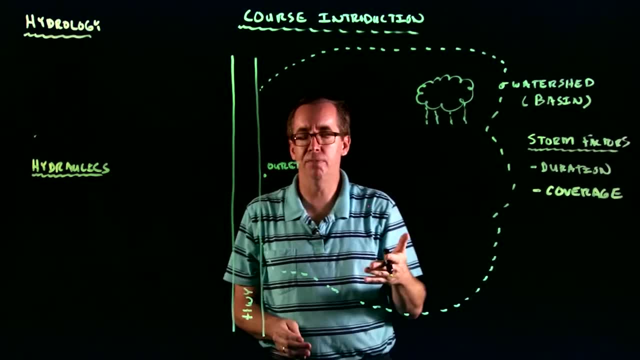 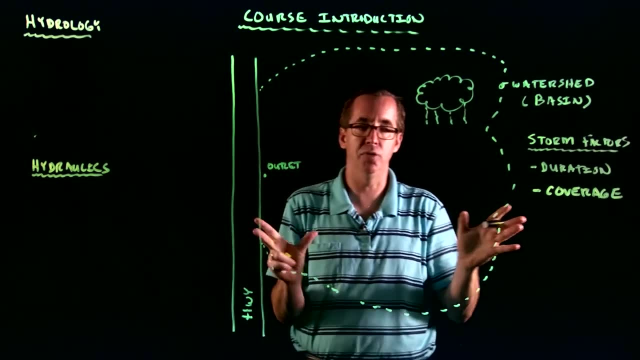 or is it covering the entire watershed, For example? you know, think when you've been on a highway and you're driving along and you're in a driving rainstorm and then all of a sudden it's like you cross this magic barrier and there's no rain whatsoever. Okay, And so that's. 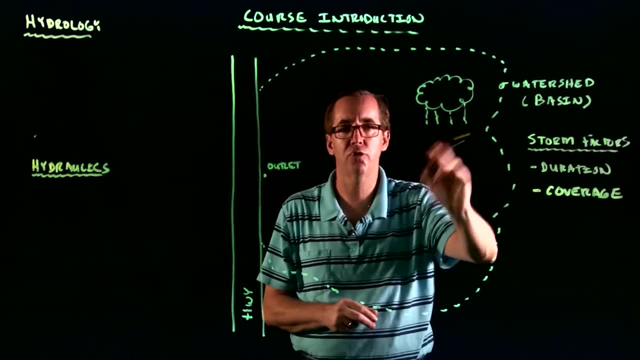 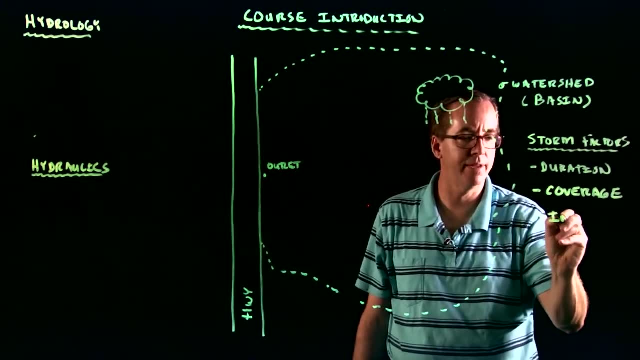 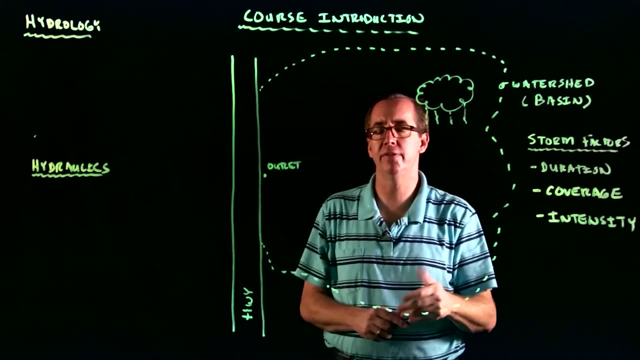 actually a huge factor is if we have precipitation in the entire watershed or just covering a portion of it. So the coverage is a big thing. The other issue that we think about is intensity. Okay, Now with intensity, what we're talking about is the difference between the storm. 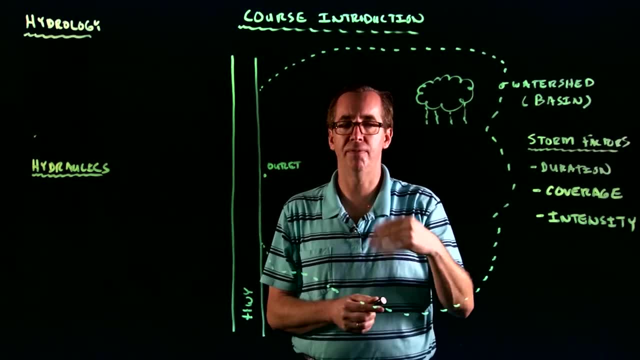 that say, say, you start off with a few raindrops, you're out for a walk, you feel a few raindrops, and then little by little it builds up and then it's a really strong storm and then it kind of 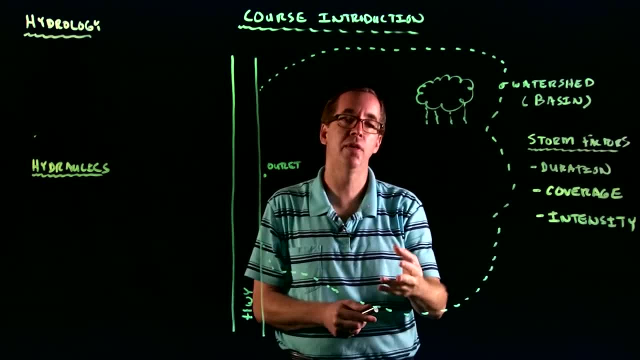 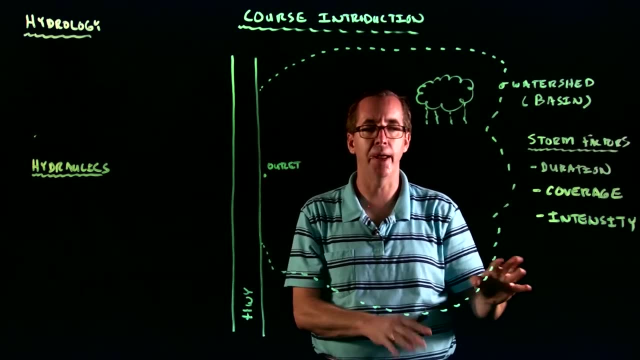 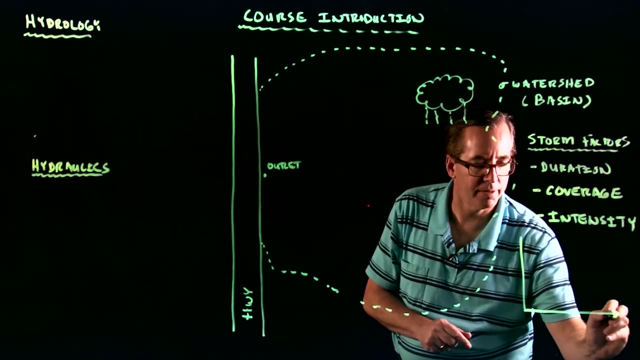 peters out Versus another storm which is common here in the south, in which without little, with a lot of water doesn't last very long and then just kind of fades away. So that's what we mean by intensity And we actually plot this. we can plot, sorry about that. let's see if we plot time. 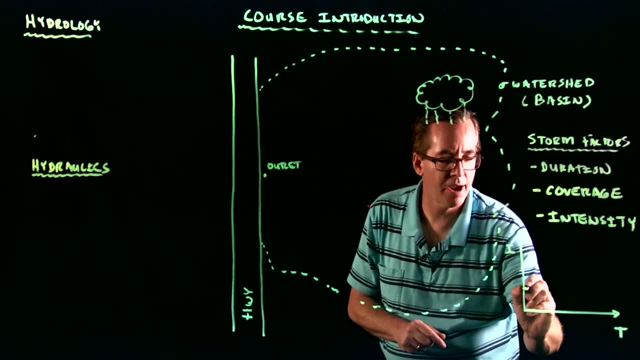 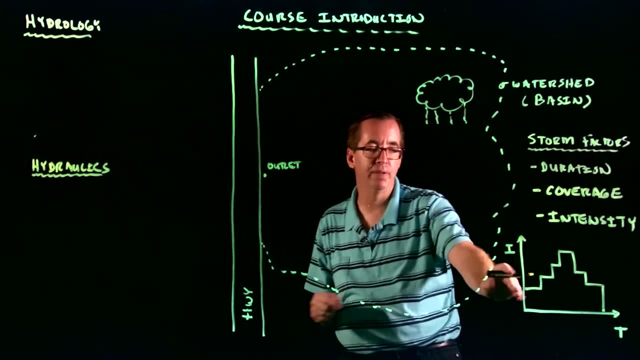 versus intensity. we might get a graph that looks something like this. It's usually a type of histogram And again each one varies in terms of its shape. You know, in this particular one you can see there's a gradual buildup. it reaches a peak and then kind of drops out. 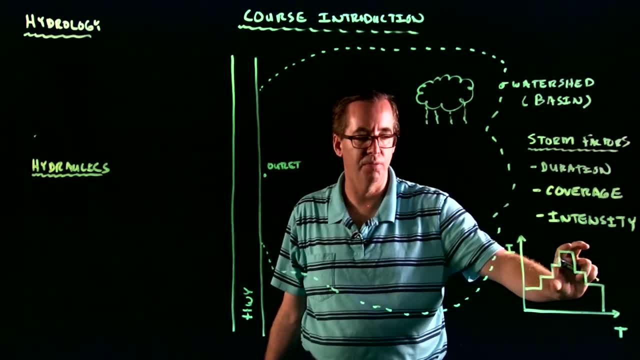 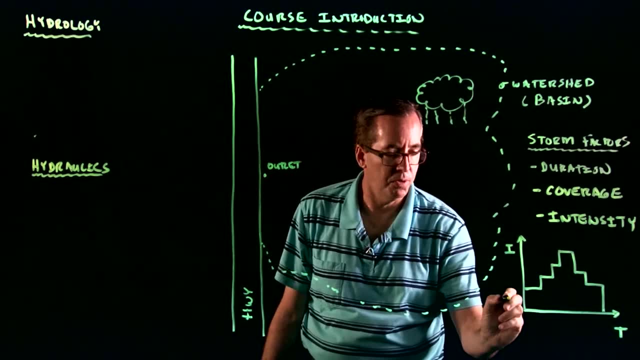 Some might have an intensity that's really strong at the beginning. some might have an intensity that's really strong at the end of the storm. okay, This graph here we actually refer to as I'm going to do the line here. this is referred to as a hiatograph And we're going to learn a lot. 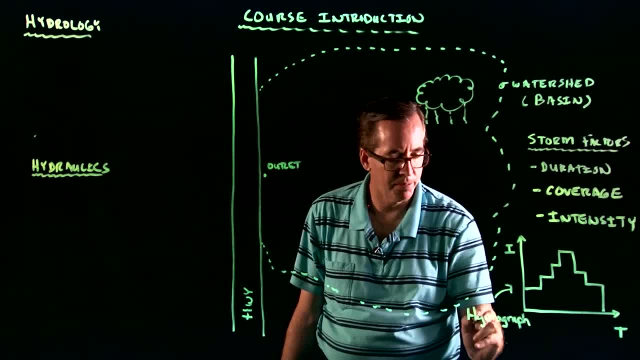 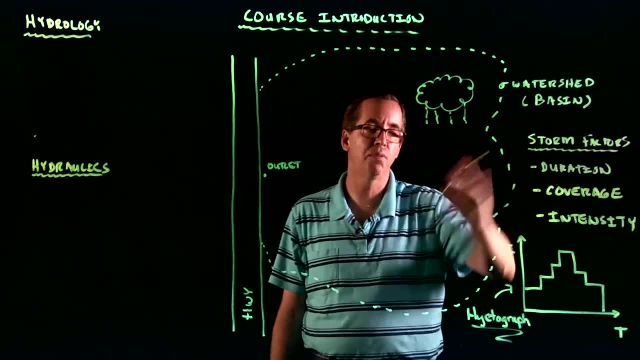 about these in class. So right now I'm just kind of sharing with you some of the technology or some of the terminology. okay, That's a hiatograph. Okay, so that takes us actually through the first part of the course, So in hydrology, a good portion of the course. 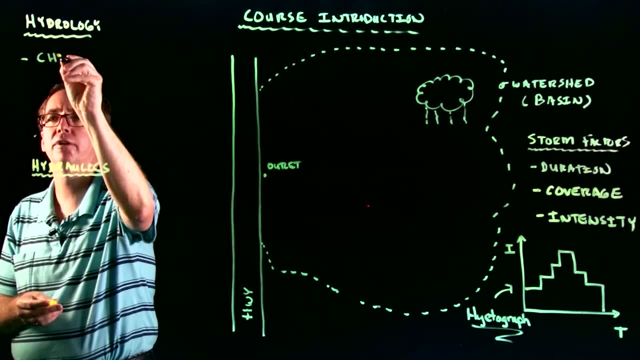 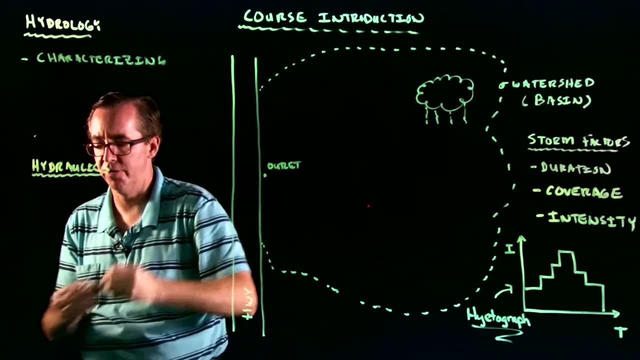 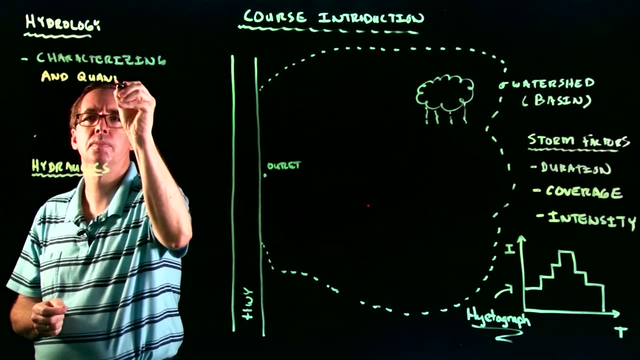 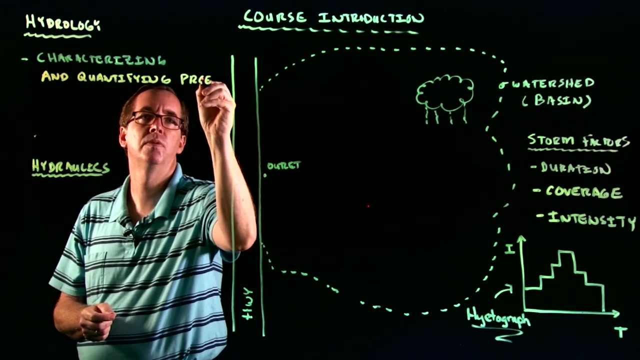 the course is focused on what we on either characterizing- let me switch markers here- this one's getting a little low in quantifying rainfall, Okay, and I'm just going to say precip, Oops, precip, Try that, I don't know how to erase that. 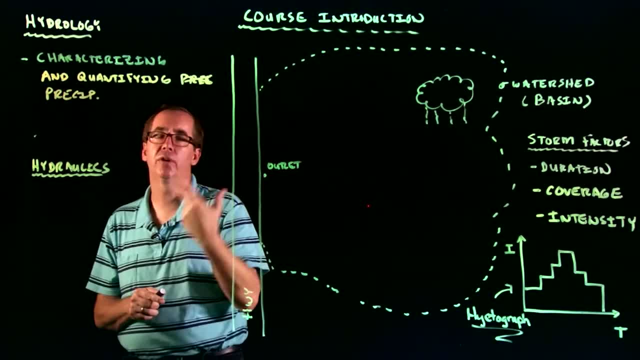 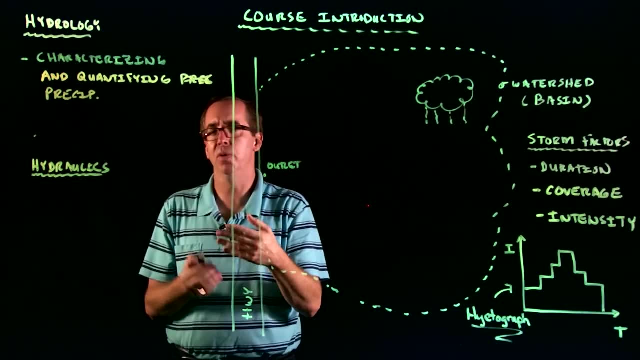 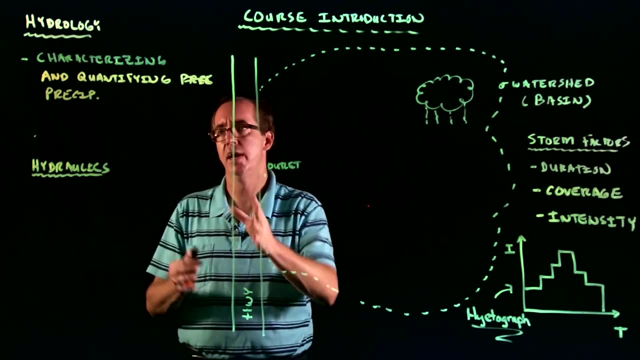 All right, so quantifying or characterizing precipitation: okay. So, essentially, how much did it rain And the rain that occurred last night was that significant of like a five-year rain event? Was that a 10-year storm? We've all heard about these periods of storms And that's. 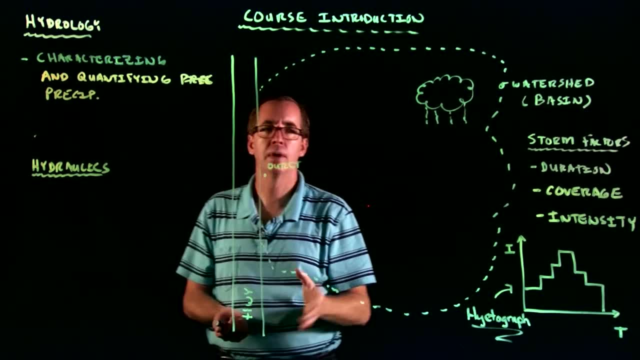 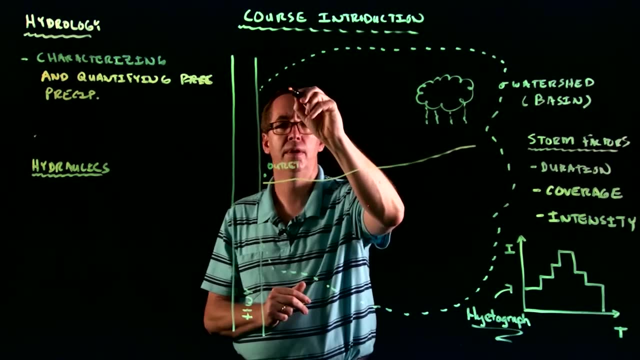 what we mean by characterizing or quantifying precipitation. Now let's look at the watershed. Now, of course, within the watershed, it's likely that we're going to have several streams, right, And they're going to have different branches, okay, And again, all this flow eventually is going to make its way. 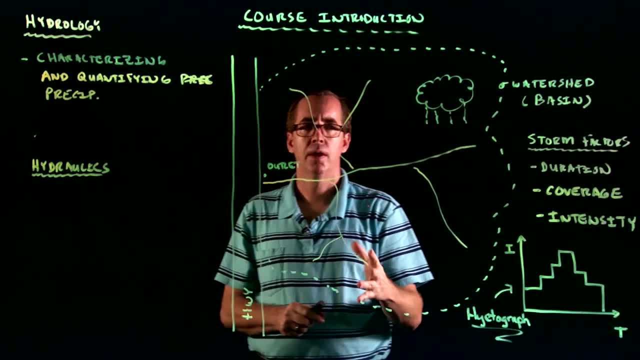 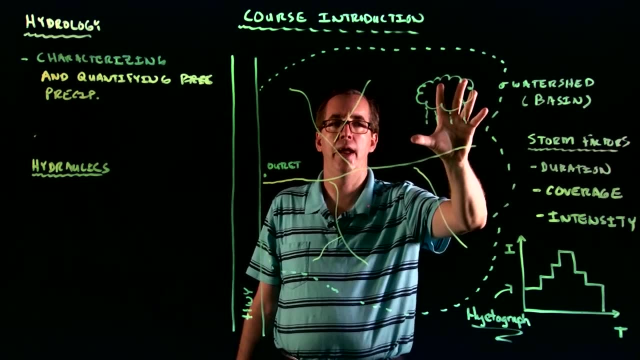 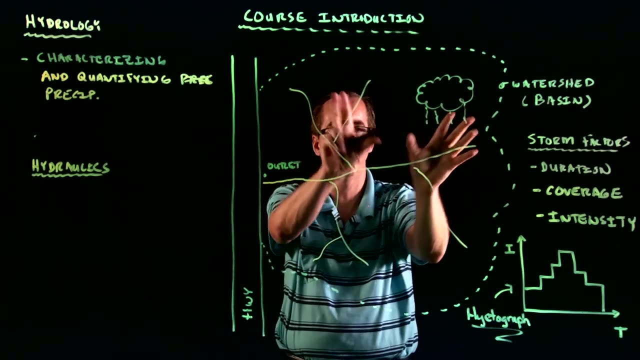 to the outlet Say: we have a storm Now. initially maybe the storm starts over here in the northeast corner of the watershed, And initially maybe this is: it gets saturated and then, little by little, parts of the watershed start contributing to the flow. 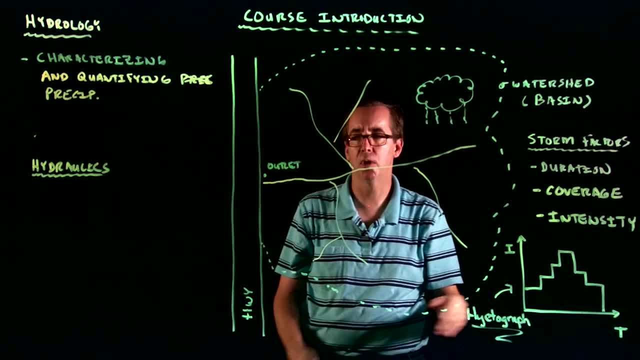 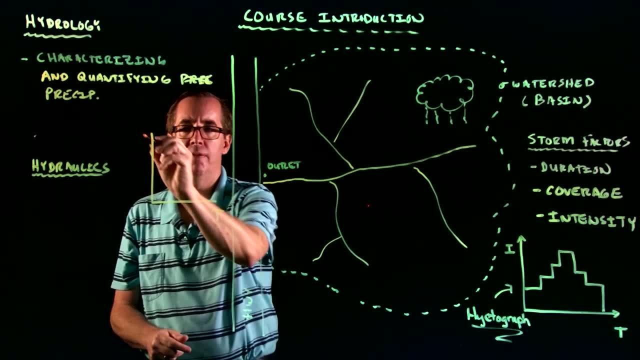 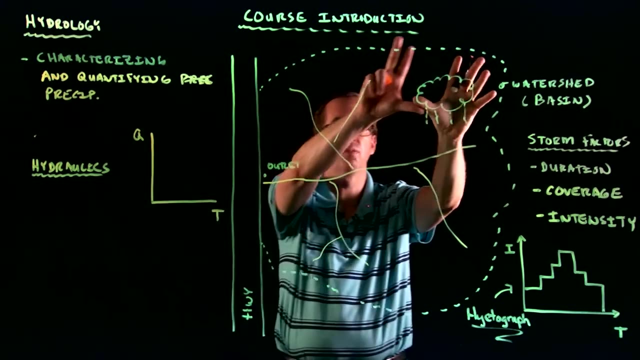 And eventually all the flow is going to make its way to this outlet, okay. So if we actually look at that outlet, if we actually plotted that over time, we have a flow over time, okay. And so again, initially maybe this part gets saturated and then the runoff. 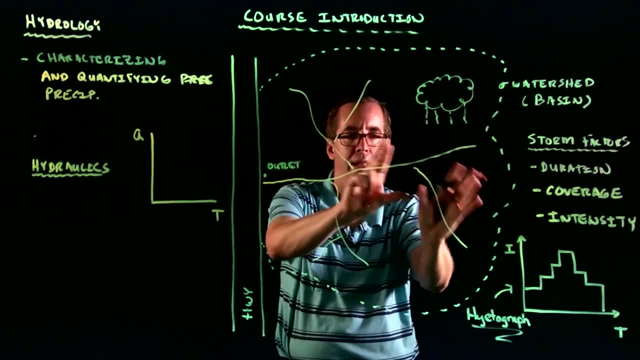 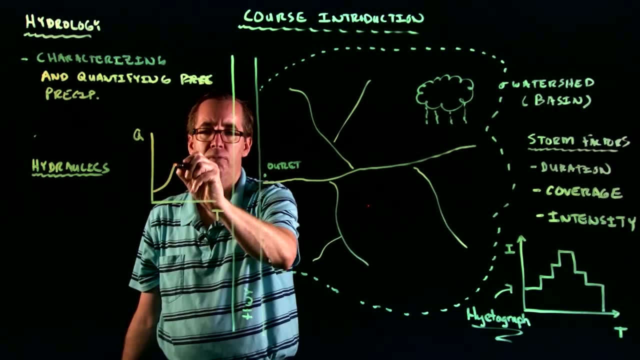 from here starts making its way down, and these rivers start contributing, And little by little everything contributes. And so at this point here, if we actually had a flow meter, it would actually register the flow going through that outlet And again it would pick up. 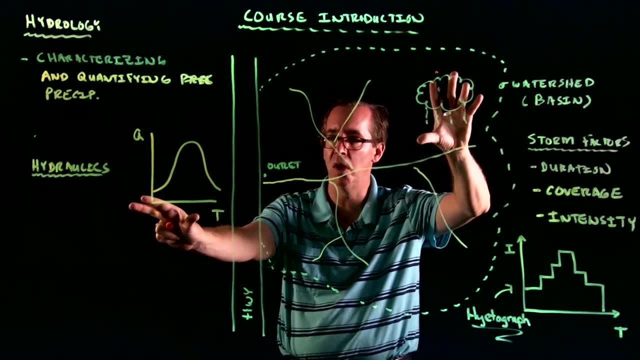 it might start off real small because there's not a lot of flow And so, at this point, a lot of areas contributing to the flow, But little by little it's all contributing. It reaches some peak flow And then from that point on it's going to drop off once the storm. 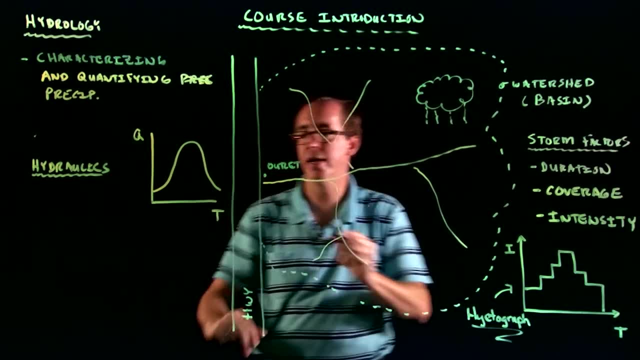 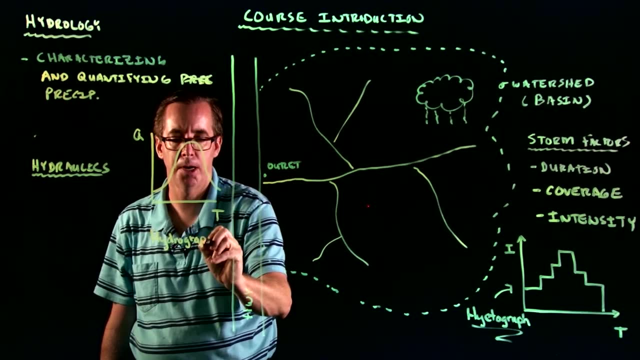 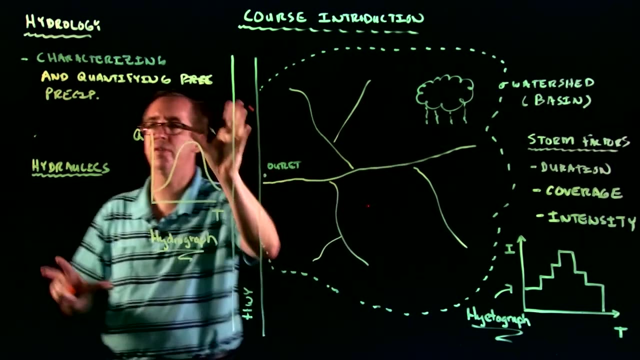 eventually ceases. okay, This right here is what we refer to as the hydrograph Hydrograph. okay, So that's the second part of the class in terms of the hydrology component is the first part is characterizing the rainfall And the second part is understanding. 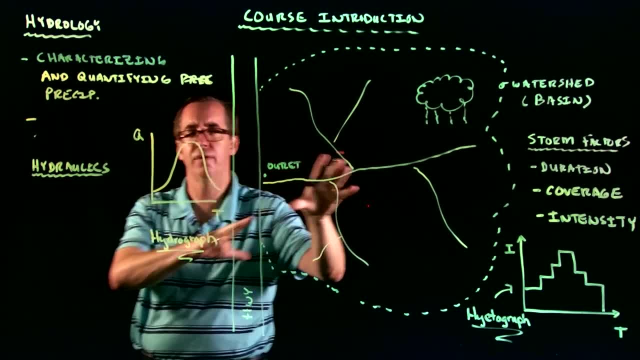 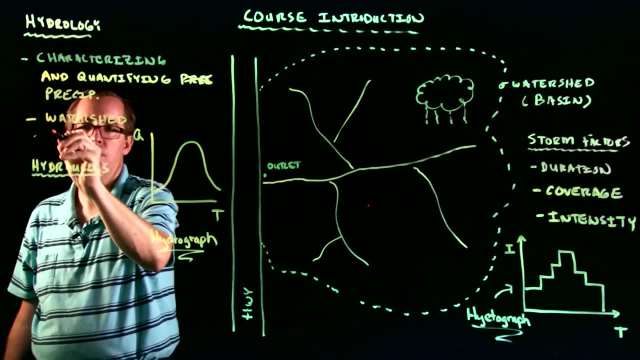 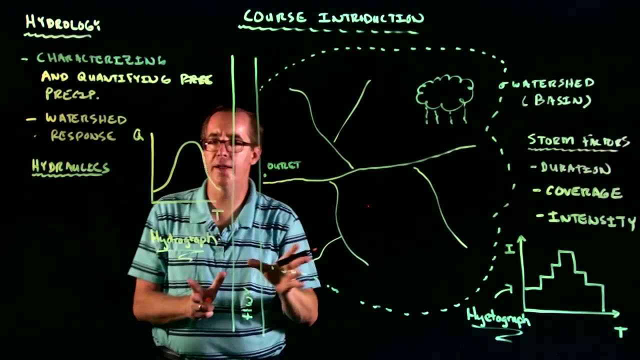 how the watershed's going to respond to that rainfall. So say, watershed response. Okay, And again, there's a lot of factors that contribute to the watershed response. We're going to talk about those in more detail. I'm not going to put them up on the board. 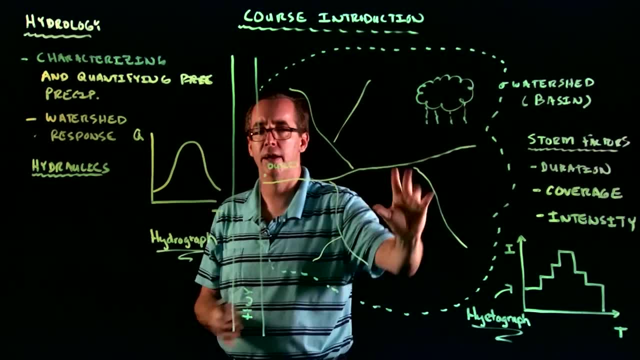 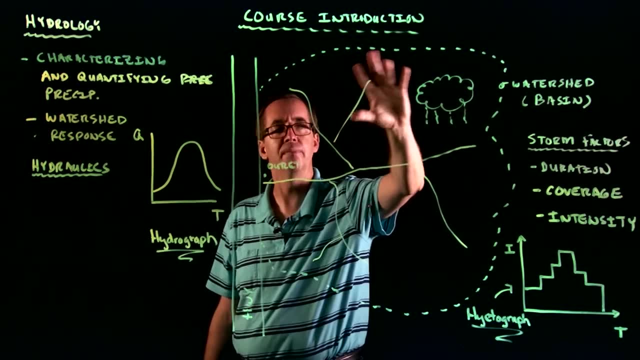 but you can imagine. some of them are the obvious, like the size of the watershed, the slope, you know. Is it a watershed response? Is it a watershed response? Is it a watershed in an area that's like a farmland, that's flat? Is it a watershed with a lot of mountainous areas? 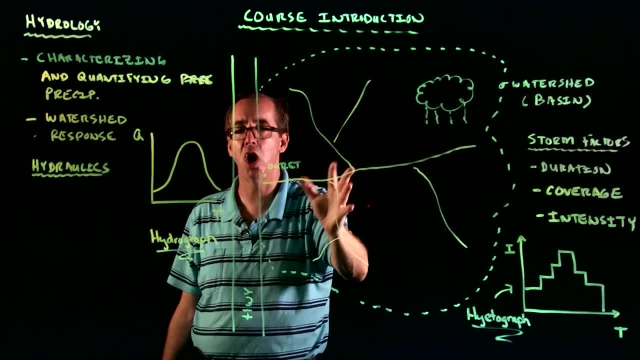 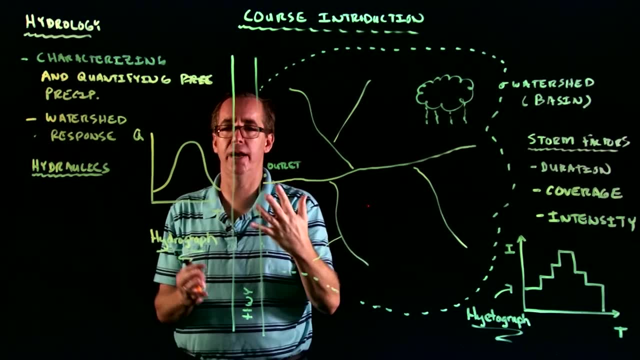 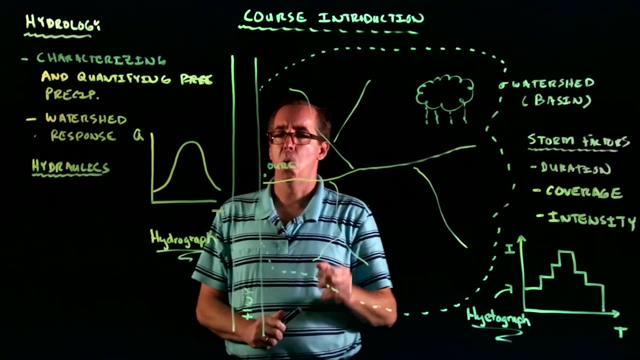 where the slope is steep and that would influence a lot: the runoff, the vegetation cover, the type of soils that we have, the condition of the soils. There's a lot of factors that go into that. Now let's talk a little bit about the hydraulics component of this course. okay, With the hydraulics. 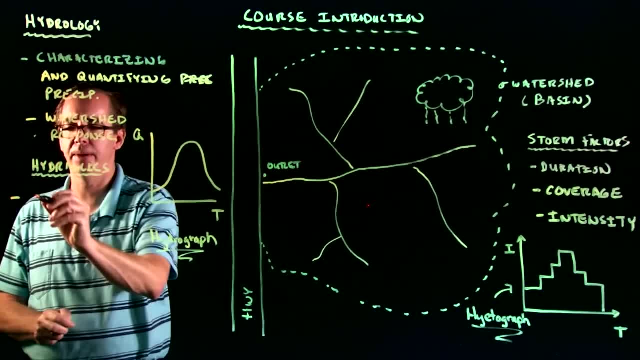 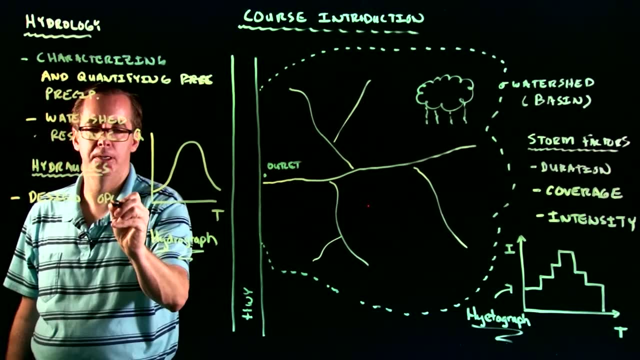 part, the main part of the course in hydraulics. what we're talking about in hydraulics, basically, is the design of the watershed. So what we're talking about in hydraulics is the design of the watershed. So we're talking about the design and operation of structures used to control this. 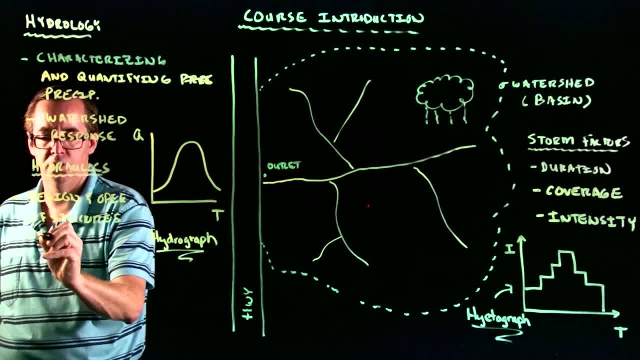 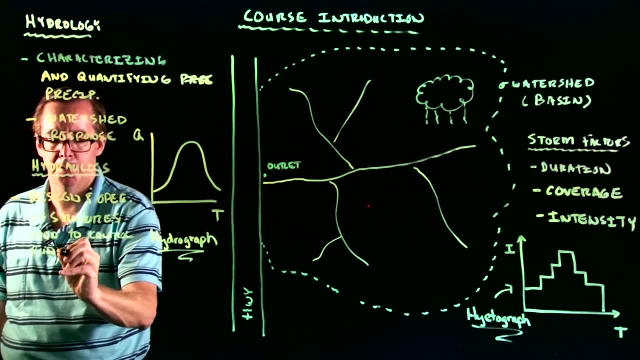 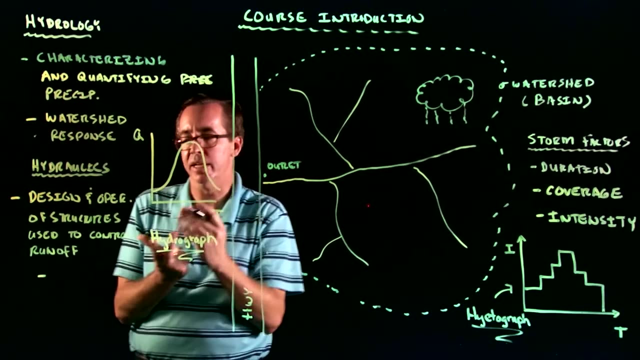 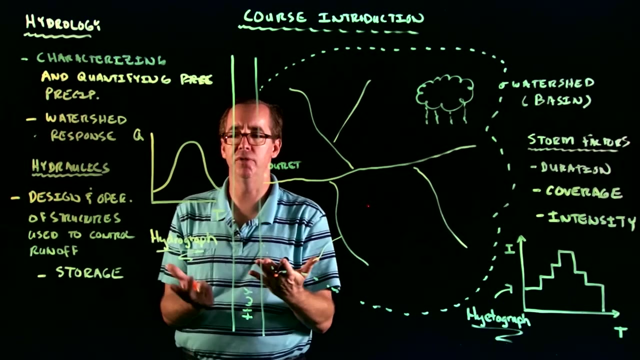 runoff of structures used to control runoff: okay, And these structures could vary. Some structures are aimed at containing them or storing them, So we have storage, storage type of structures. okay, Examples of these would be detention ponds, retention ponds. 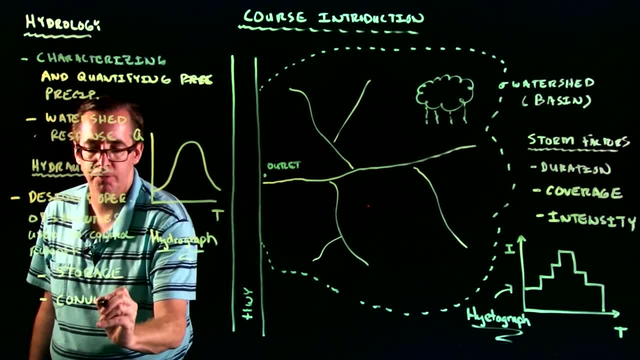 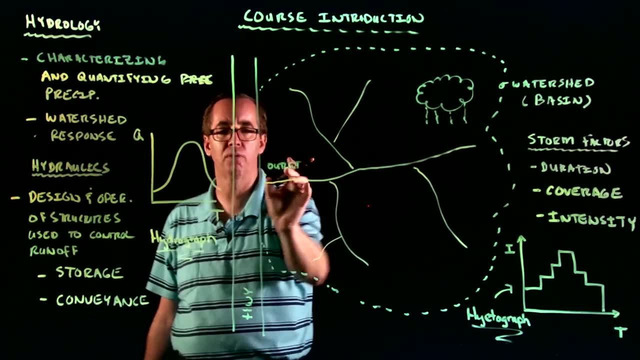 Some are used to convey water, okay, So we say conveyance, okay, Conveyance would be an example that we have here in this diagram. So we have all this water arriving to this one point and we have a highway. Wow, well, there's going to be an issue unless we build some type of hydraulic structure. 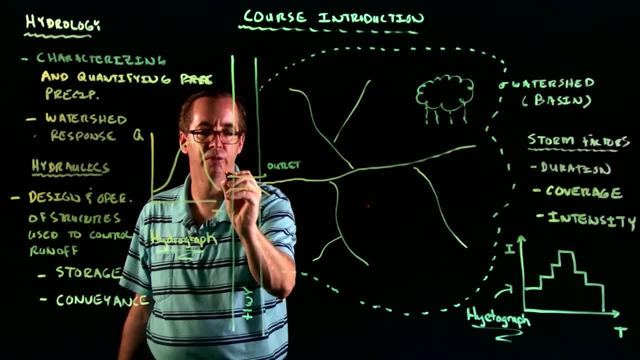 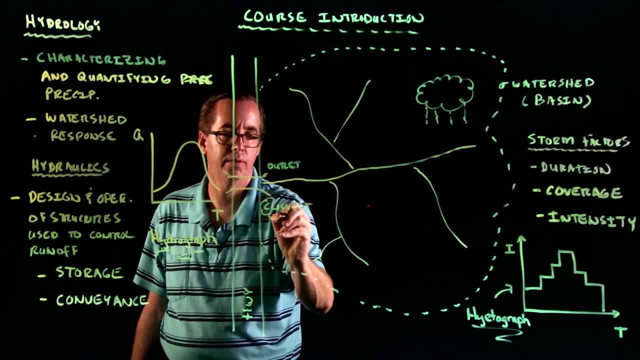 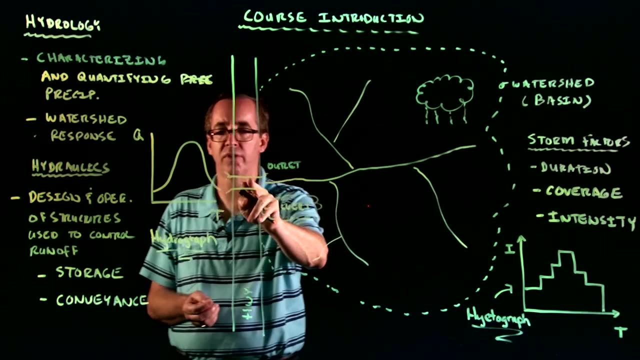 And that hydraulic structure, in this particular case, would be a real common one called a culvert. Okay, so I'll do that. So we've got a culvert. okay For us to design this culvert. clearly, we're going to need to know how much flow that we're expecting at this point so that we can design it. 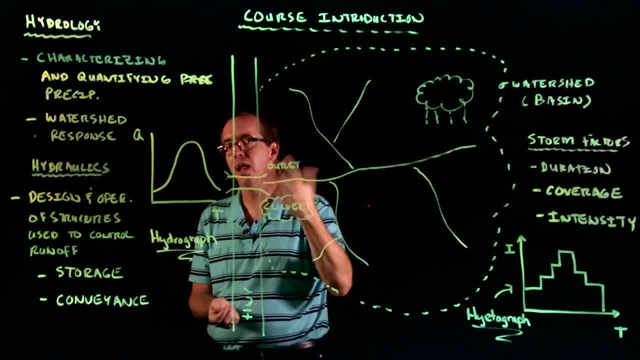 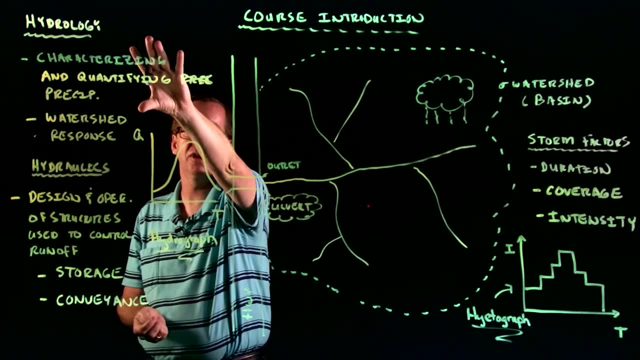 so it can pass all this flow, okay. And so the hydrology part is used to tell us how much water we expect to get, based on the watershed response and based on the characteristics of the storm itself. The hydraulics part is: how do we design? how do we design, how do we design the flow of the 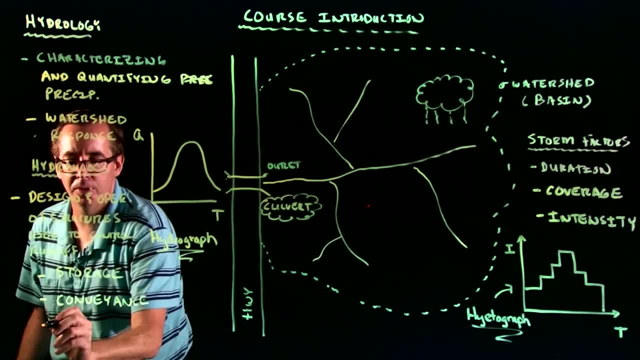 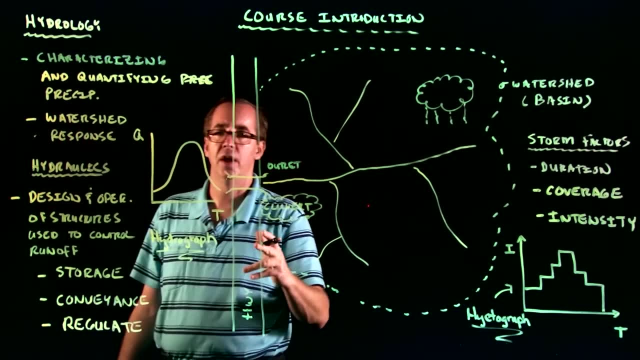 structures that can either store water, convey water. Sometimes we want to regulate water. For example, we spend a lot of time in this course with regulation structures that are used in irrigation applications, when we have so much water and we want to divvy it up so many gallons per. 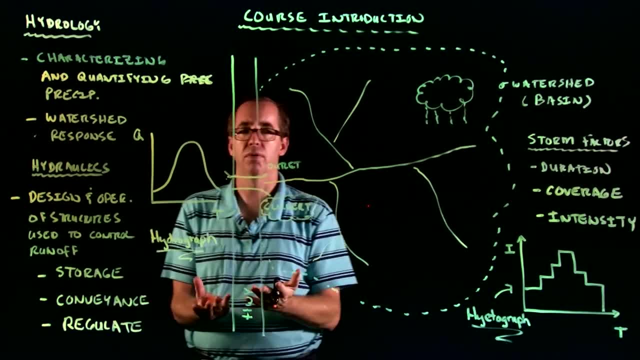 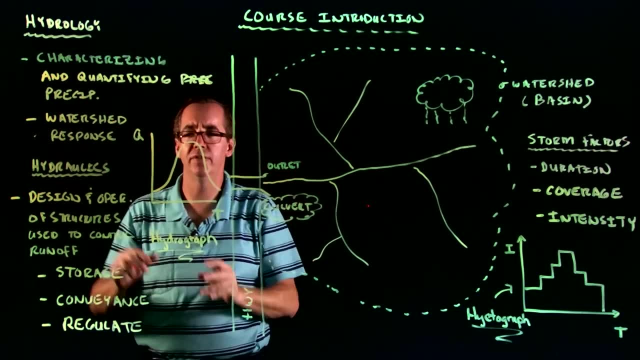 minute to this field, so many gallons per minute to this field, and so forth. okay, So that concludes this video. Again, the highlight of this video, the most important part, was A. we defined what hydrology is and what hydraulics is in a common 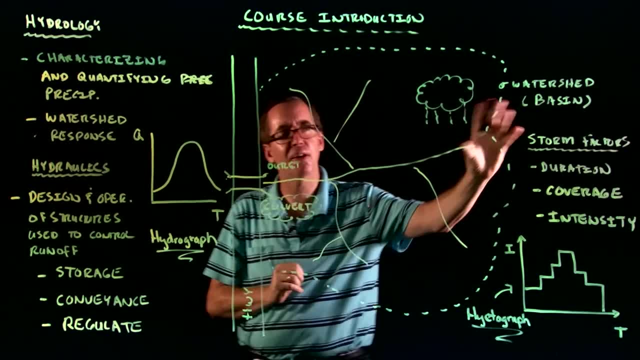 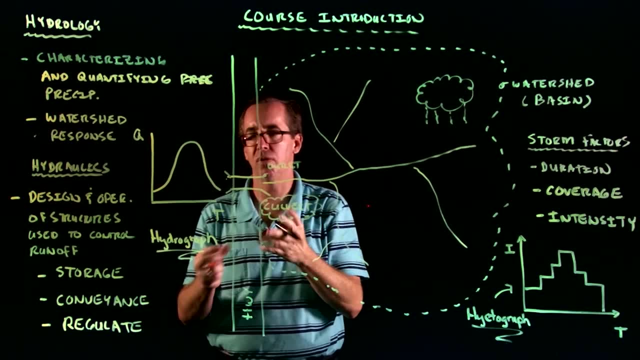 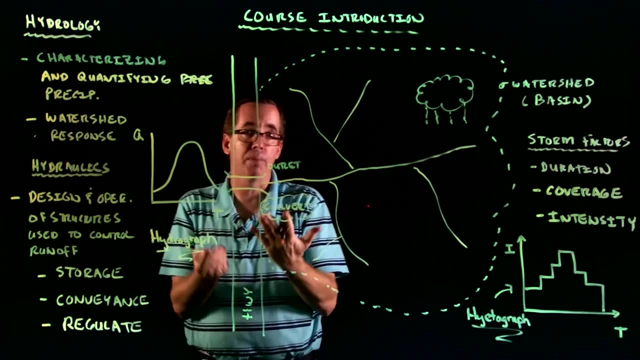 everyday type of application. We talked about some of the factors that influence the storm variability. We talked about some of the factors that influence the amount of runoff that we would expect, and then we also talked about the type of information we would use in the hydraulics portion of the course so that we could design, in this case, a culvert or it could. 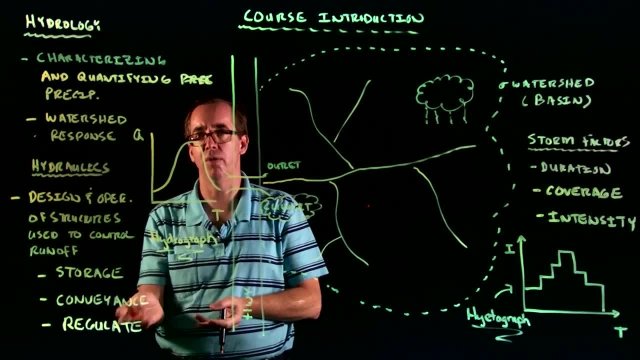 be a similar type of structure, either for storage, conveyance or regulation. Thank you so much.